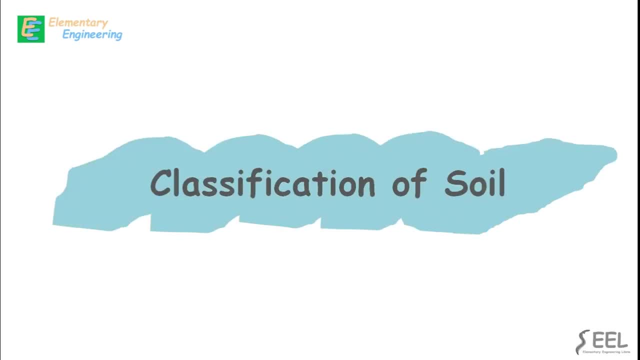 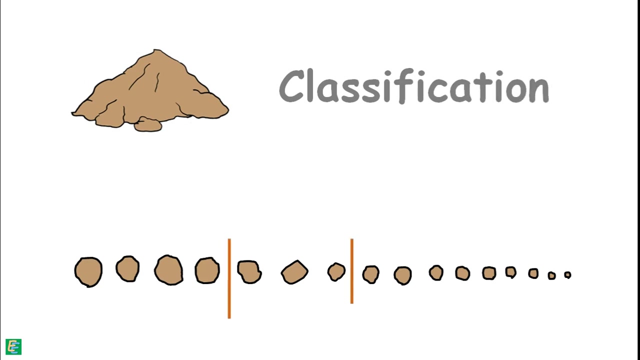 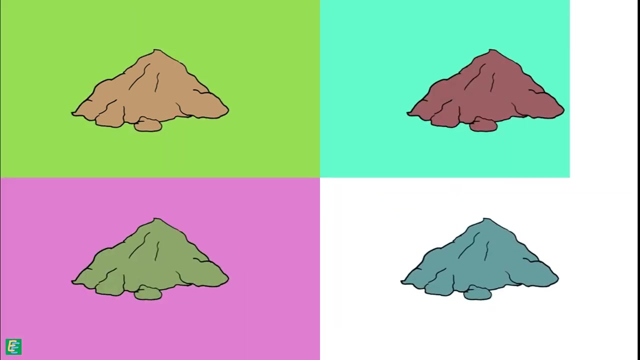 There are numerous amounts of soil present on the surface of Earth, each containing soil particles of different sizes, shapes and composition. If we classify and categorize soils, it will be convenient for us to study them. We arrange the soils into different groups, such that 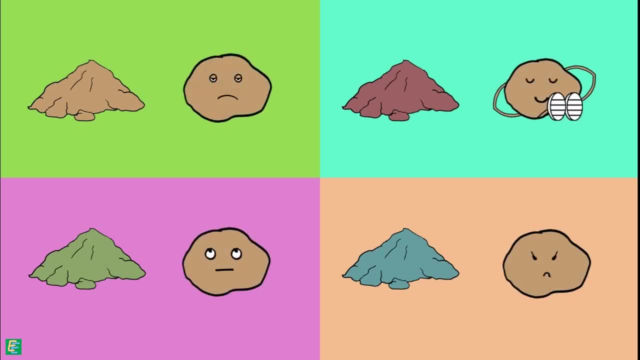 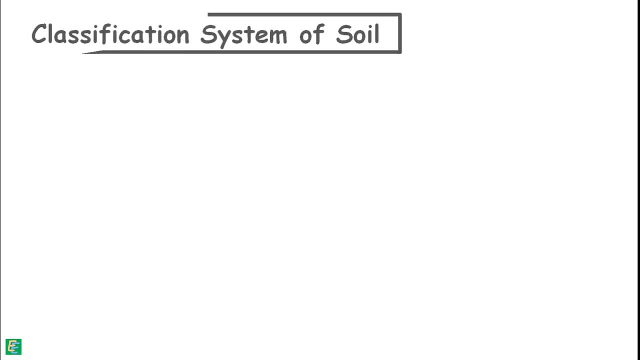 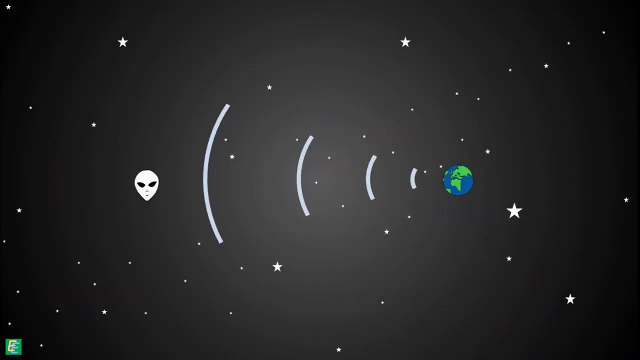 soils in particular group have similar behavior. This arranging of soil is called classification system of soil. Any classification system must provide us the information about the expected engineering properties of a soil. It works as a language of communication between engineers. Classification is done so as to convey the same meaning universally: An engineer 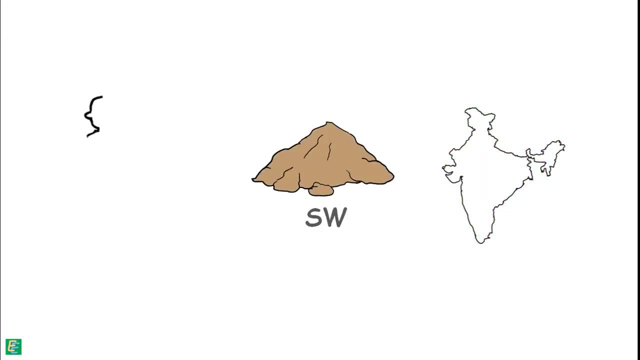 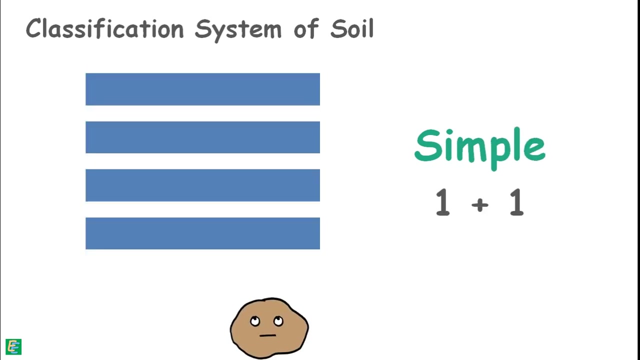 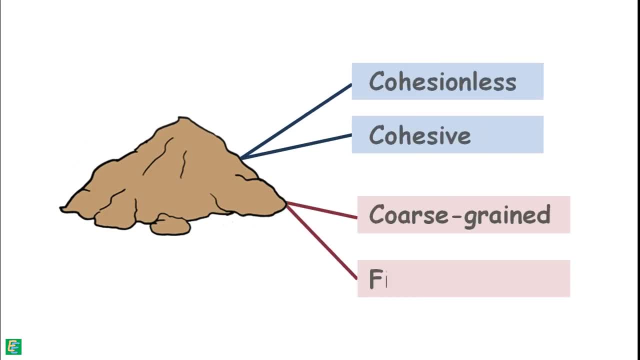 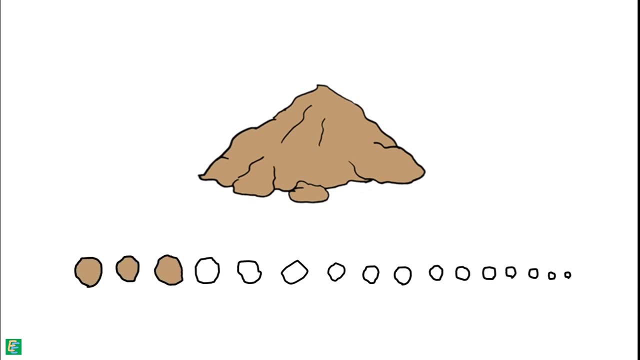 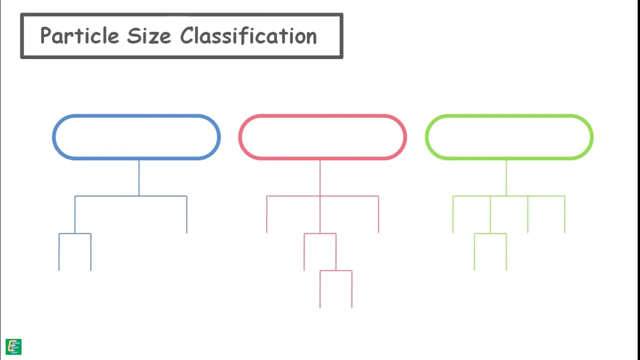 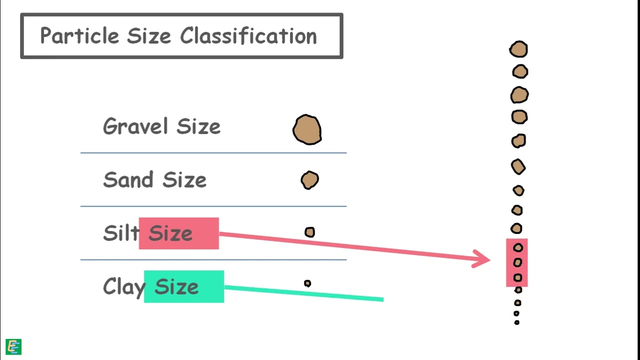 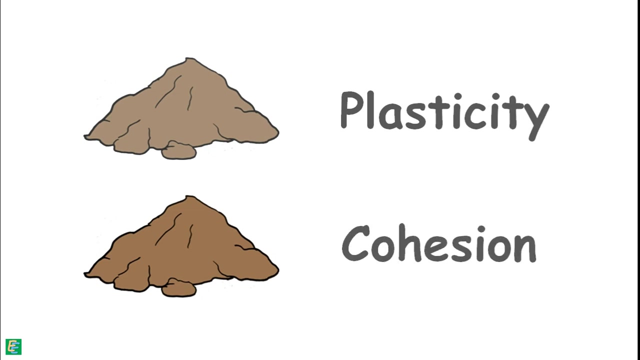 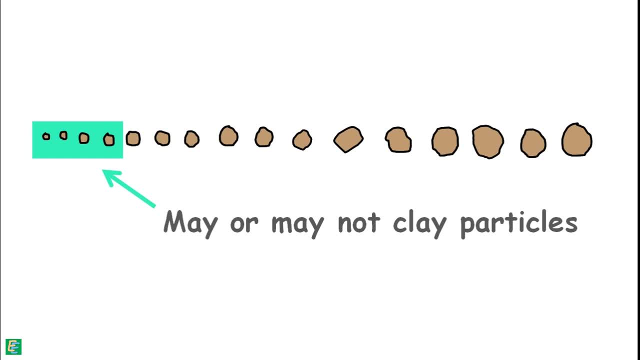 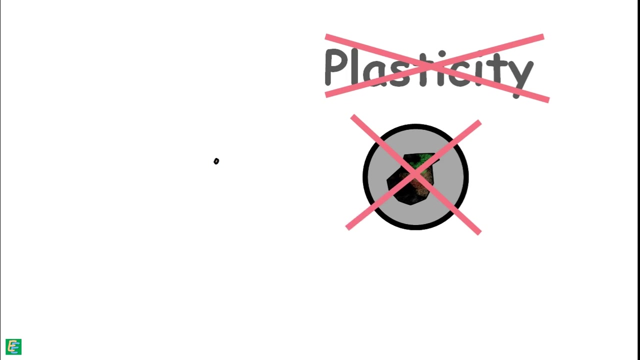 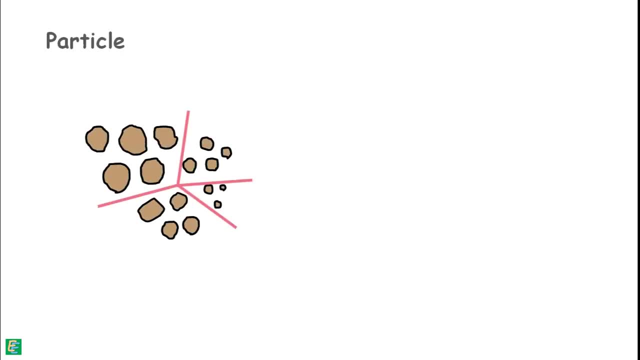 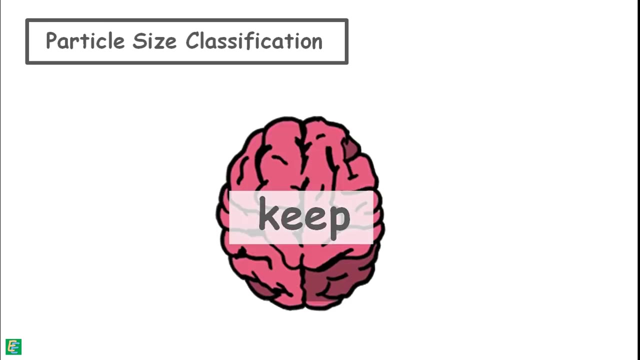 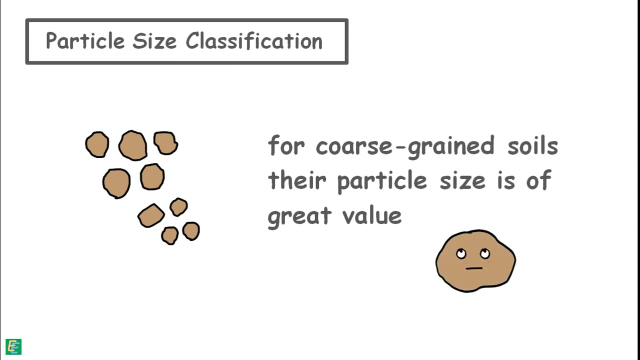 we notice, a system of soil classification purely based on particle size may be misleading, particularly for fine-grained soils, as their behavior depends on the plasticity characteristics, not on their particle size. but we must keep in mind that for coarse-grained soils, their particle size is of great value, as their behavior primarily depends upon it. these are some. 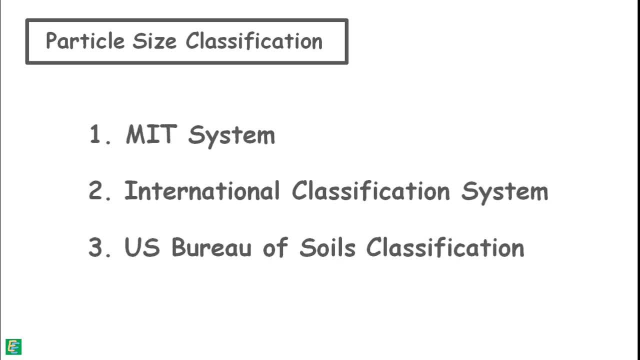 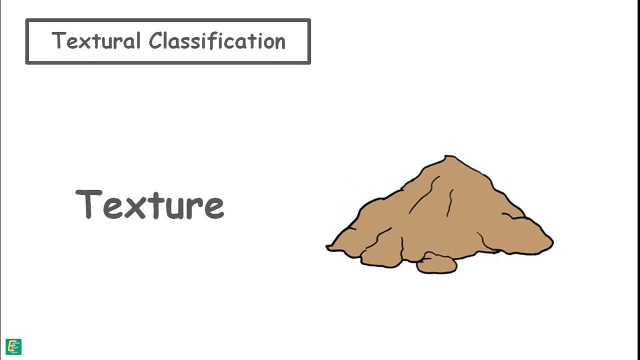 classification systems based on particle size only soils are also classified based on their texture. texture of a soil means how a soil visually appears and feeds. texture is influenced by the size, shape and gradation of soil particles in a soil. a triangular representation of textural classification system was 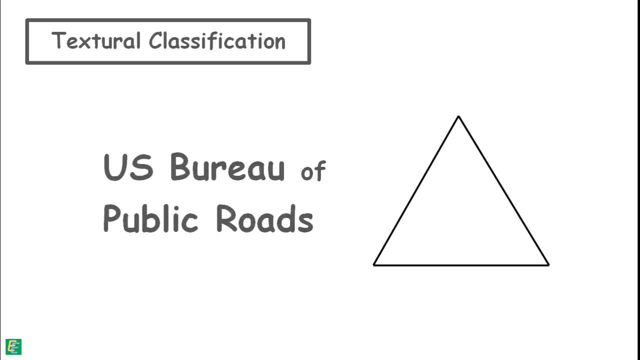 suggested by US Bureau of Public Roots. in this, the term texture is used to express the percentage of the three constituents of the soil- sand, silt and clay- on the three sides of equilateral triangle. this system assumes that soil does not contain the particles of size larger. 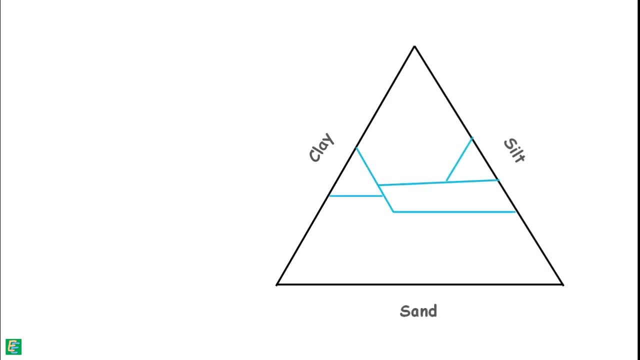 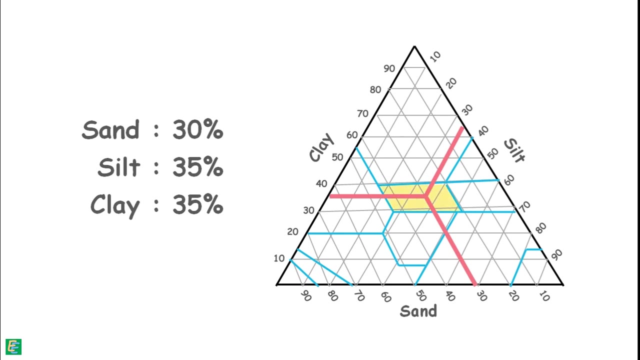 than sand. this equilateral triangle is divided into 12 zones. each zone indicates a type of soil. if we know the percentage of sand, clay and silt in our sample, we can calculate the percentage of sand, clay and silt in our sample. we can use this triangle to know our soil type out of these 12 soil types. 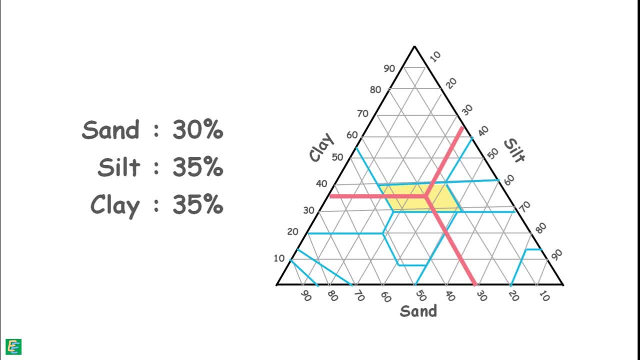 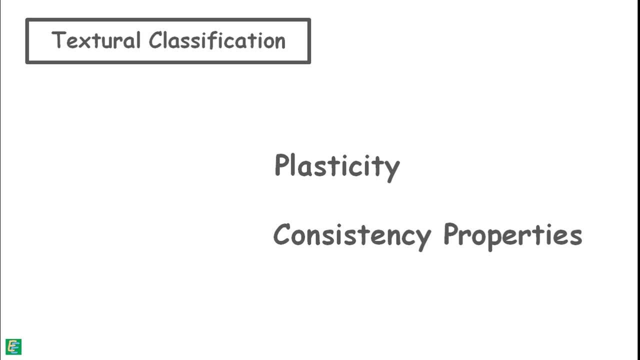 classified in the triangle. but this system also does not takes into account the plasticity and consistency properties, which are important when it comes to the fine-grained soils. two classification systems- unified soil classification system and AASHTO- are adopted by US engineering agencies and state departments. other countries in the world, such as the United States and the 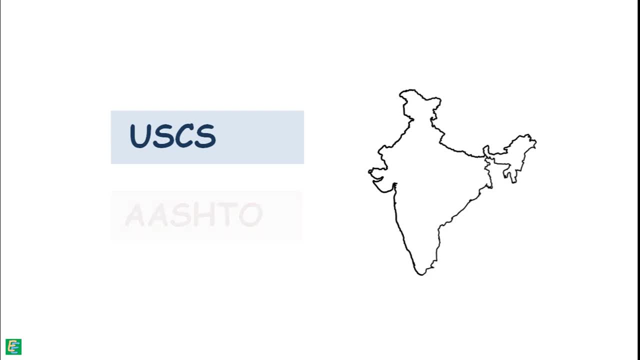 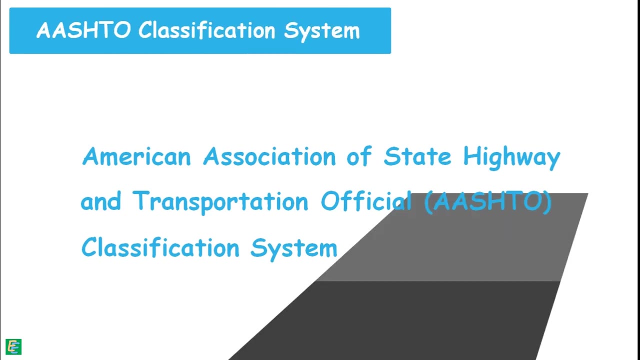 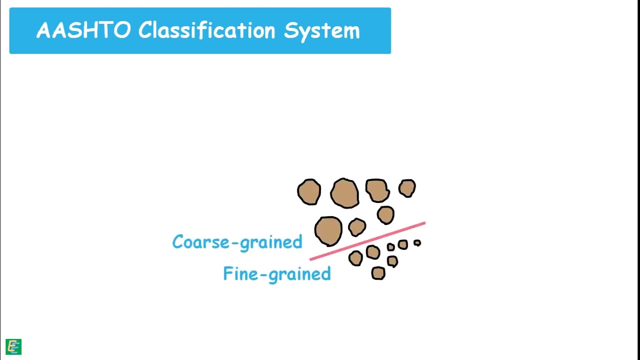 United States, including India, has also adopted the unified system with minor modifications. AASHTO stands for American Association of State Highway and Transportation official classification system. it is particularly useful for classifying soils for highways. this system classifies both coarse grain and fine-grained soils, using both particle size analysis and plasticity characteristics of soil. 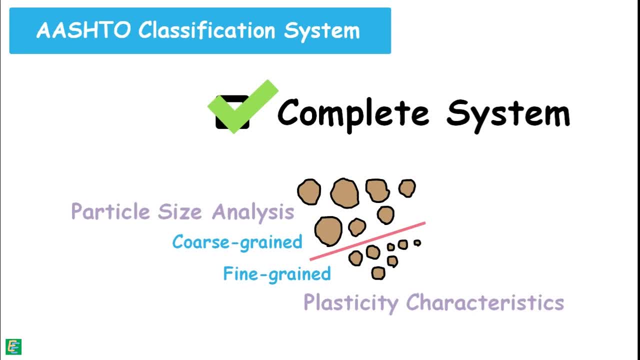 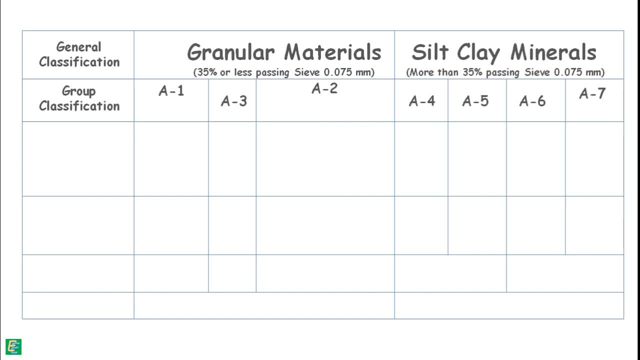 which makes it a complete classification system. In this system, soils are divided into 7 types, designated as A1 to A7, based on their relative expected quality for road embankment and subgrids. Some of the groups are divided into subgroups. 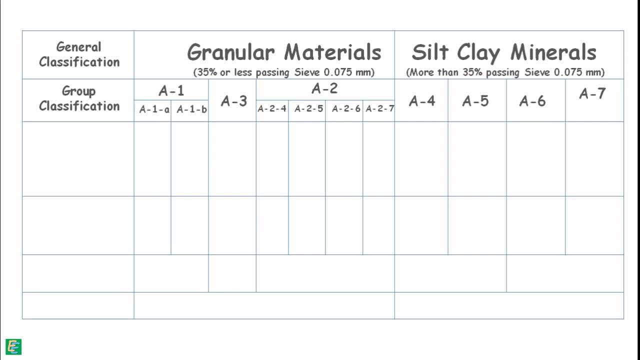 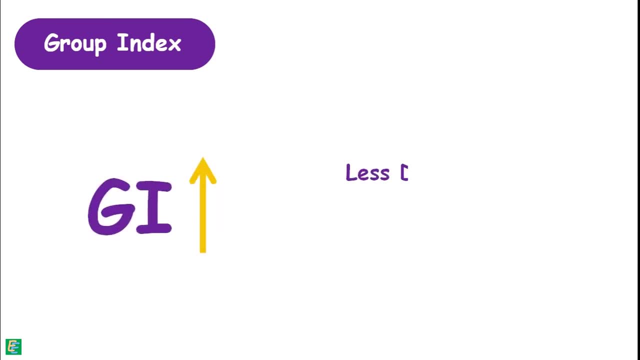 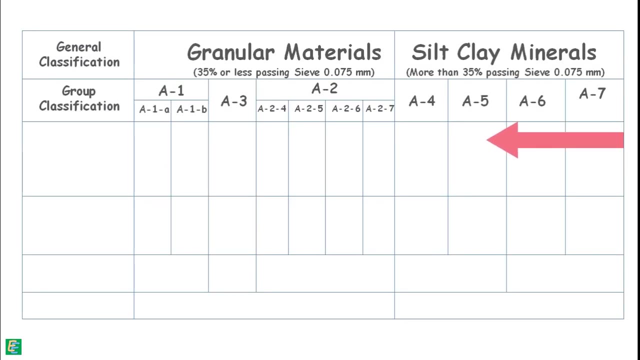 Soils within each group are evaluated according to the group index calculated from this empirical formula. In general, greater the GI value, less desirable is the soil for highway construction within that subgroup. Likewise, a soil with lower number, say A1, is more suitable for highway material than 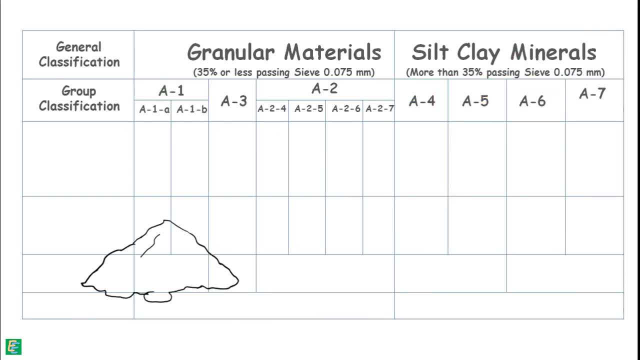 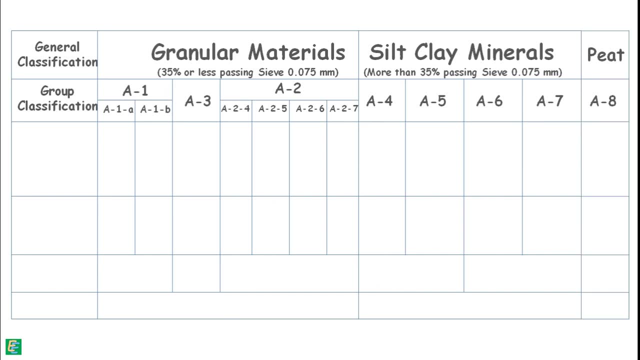 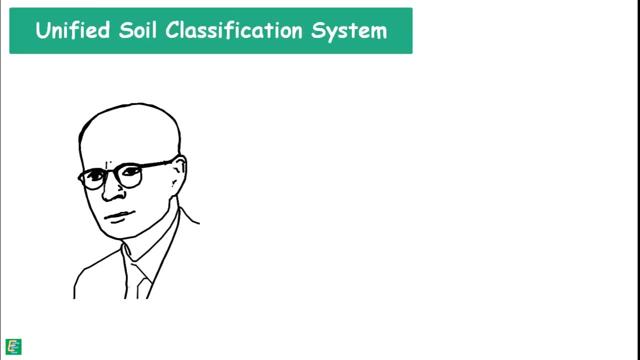 A4. In AASHTO system initially there was no place for organic soil, So additional group A8 was introduced for peat. Then comes the unified soil classification system. It was first developed by Casagrande and later it was modified by Bureau of Reclamation. 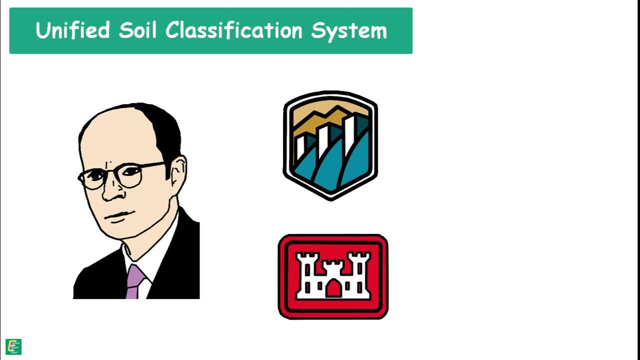 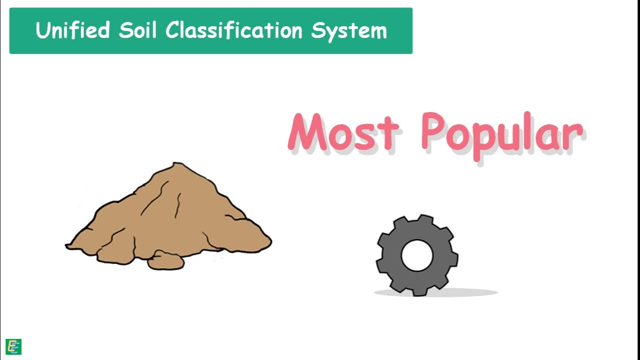 and the Corps of Engineers of the USA. This system has also been adopted by American Society of Testing Materials. It is the most popular system for use in all types of engineering problems involving soil. This system identifies soils primarily as coarse grained, fine grained and highly organic. 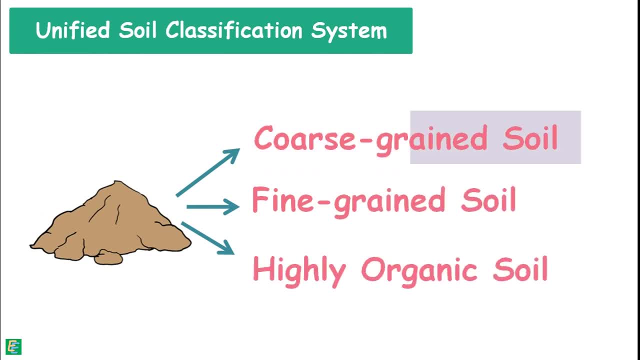 and highly organic. coarse-grained soils are classified on the basis of their grain size distribution, and the fine-grained soils, whose behavior is controlled by plasticity, are classified on the basis of their plasticity characteristics. according to this system, coarse-grained soils are those which, when 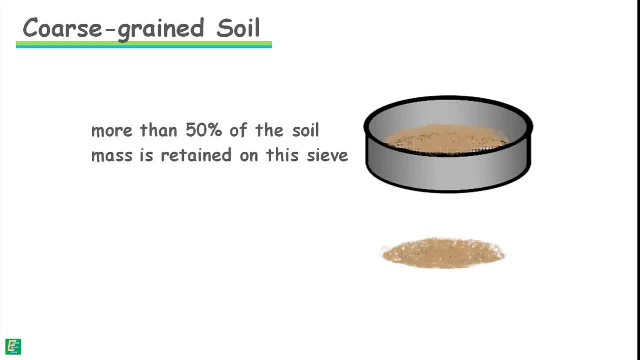 seaved, more than fifty percent of their mass is retained on 0.075 MMC. it means more than 50% of the soil mass contains particles which are larger than 0.075 mm could not pass the 0.075 mm C if more than 50 percent of the soil 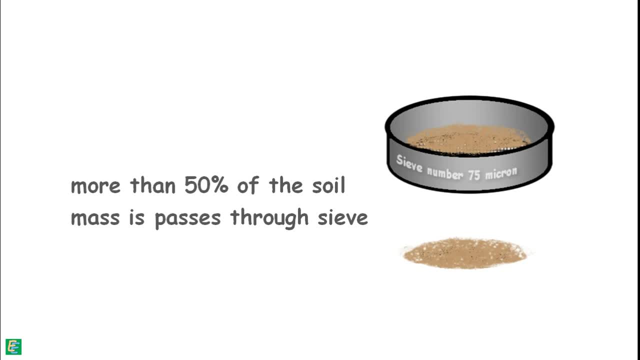 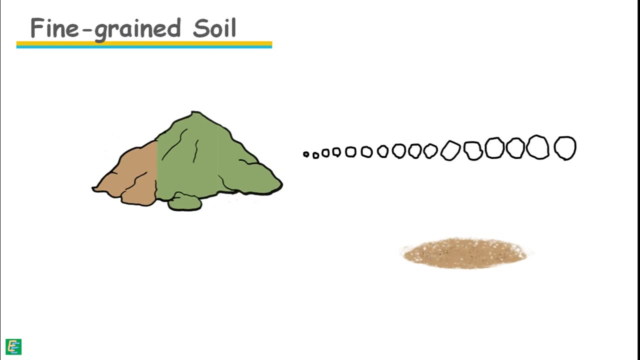 material passes through this sheave, then the soil is classified as fine-grained soil. This soil will contain contain more than 50% of its soil mass made up of particles which are smaller than 0.075m. These are some symbols used in the system to classify the soils. 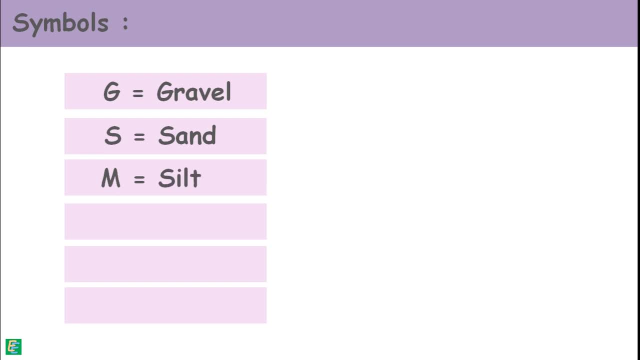 G is for gravel, S is for sand, M for silt and C for clay. O is organic and PD is for peat. Peat are highly organic soils. Peat also uses symbols W for well graded, P for poorly graded, L for low plasticity. 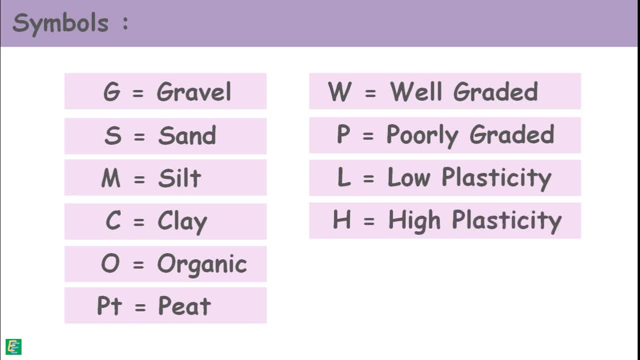 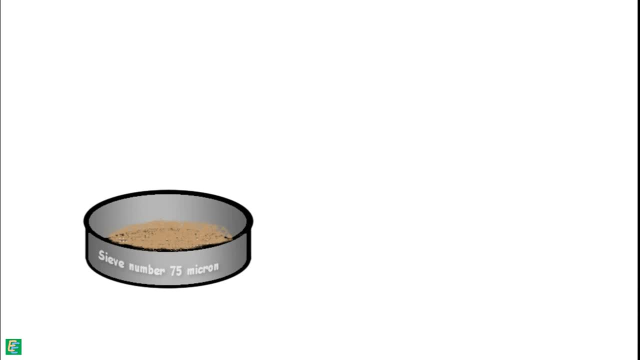 and H for high plasticity. Coarse grained soils are further divided into two categories. We further sieve our obtained coarse grained soil part using 4.75mm sieve. This sieve has larger openings than that of which we used earlier. What we are trying to do is to separate the coarser part of the coarse grained soil. 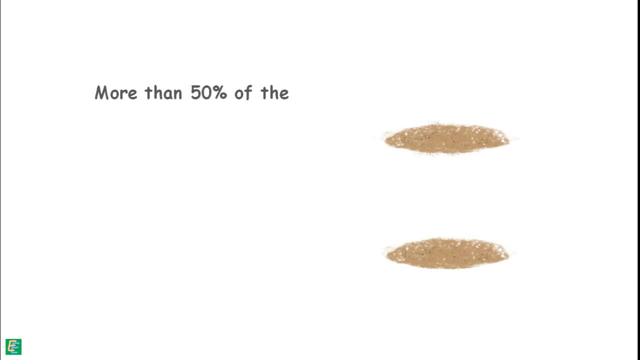 From the finer part. If more than 50% of this coarser fraction of soil is retained on this 4.75mm sieve, then soil is designated as gravel and is denoted with letter G, And if more than 50% of coarser fraction of soil passes through this sieve, soil is called. 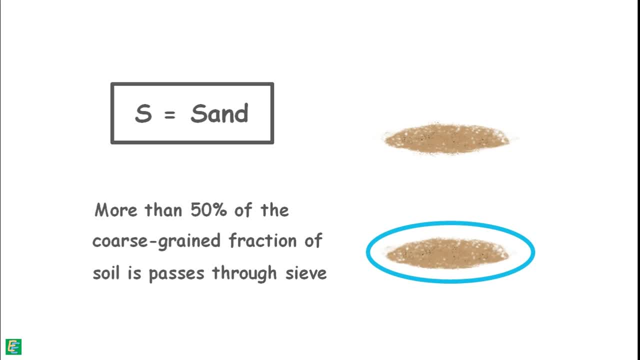 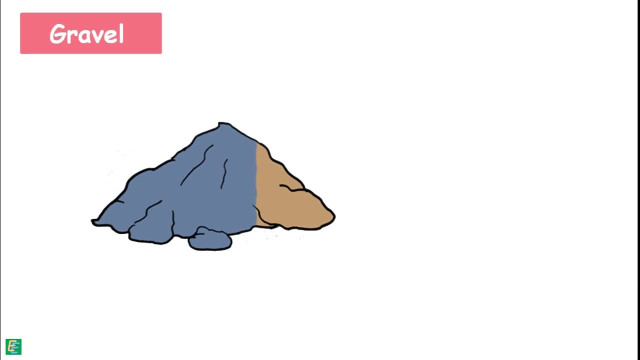 sand and is denoted with the letter S. A soil labeled as gravel has more than 50% of coarse grained particles, Which may also contain some percentage of sand particles and some of fines. If the percentage of these fines in this gravely soil is less than 5% and if the soil is well. 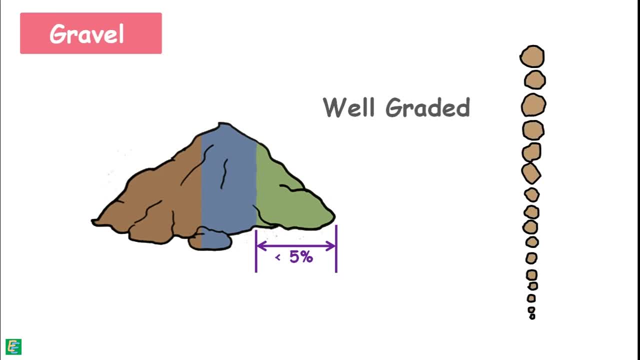 graded, that is, soil contains all kinds of soil particles, then it is classified as well graded gravel And it is represented by symbol GW. If the soil is poorly graded, then it is poorly graded gravel, But the gravel is well graded. the symbol GP. Similarly, SW and SP go for the sand. Now if the percentage of fines in the soil 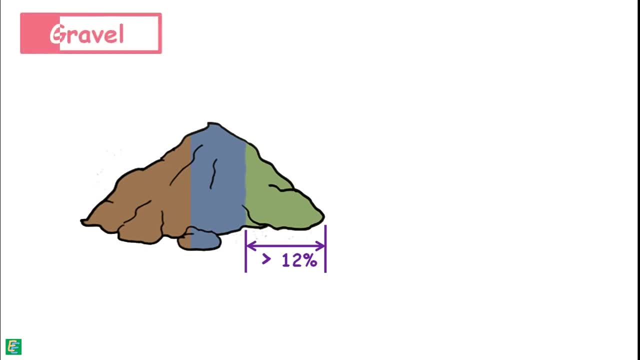 is greater than 12%, and if it is gravel soil and contains silts as its fine, it is designated as GM G for gravel and M for silt. GC if the fines are clay, SM if soil is sand and contains fines of silt, and SC if sand contains fines of clay. If the percentage of fines in coarse soils is between: 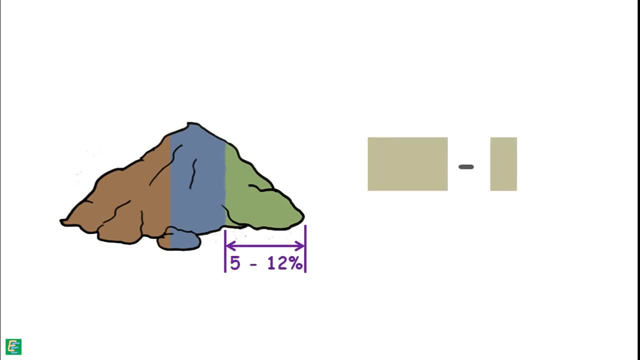 5 to 12%, then we use dual symbols to represent them. A well graded gravel having 8% of silt content is represented as GWGM. Similarly, for poorly graded sand having 9% clay content, the symbol will be SM. 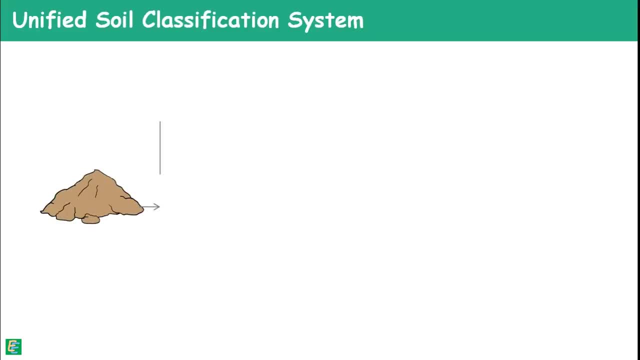 It was the classification of coarse-grained soils. Now we look into the classification of fine-grained soils. Fine-grained soils are divided on the basis of their liquid limit and plasticity properties. Casagrande plotted a plasticity chart, a graph of plasticity index of soil and its liquid limit. 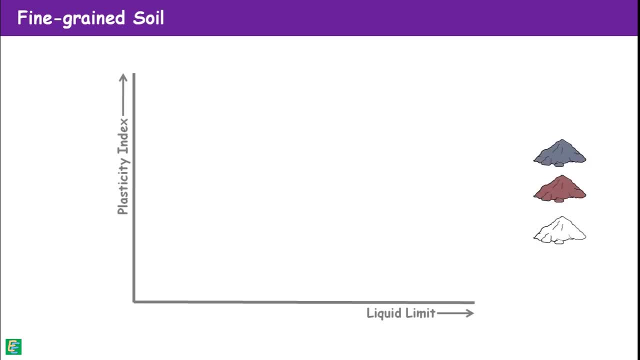 It is plotted from the experimental results of soils collected from different parts of the world. He separated clay, silt and organic soils using a graph he called A-line. Equation of this, A-line is given as this. Clay soils sit above A-line as they have high value of plasticity index. 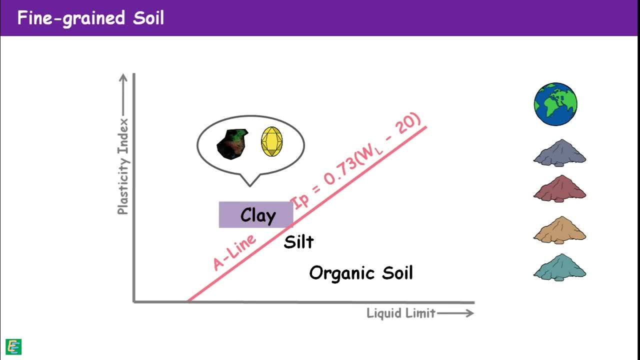 because of the clay minerals present in them, Where the silts and organic soils lies below this A-line. Let's seriously look at this experiment. trying to compute the experimental results of soils collected from different parts of the world, He separated clay, silt and organic soils using a graph he called A-line. 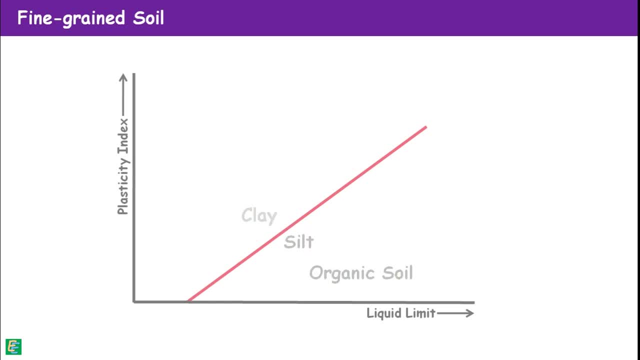 Unified system classifies fine-grained soils in two categories, as soils having liquid limit less than 50% and soils having liquid limit greater than 50%. So in the graph we plot a vertical line at liquid limit 50%. According to this system, fine-grained soils lying to the right of this line have high. 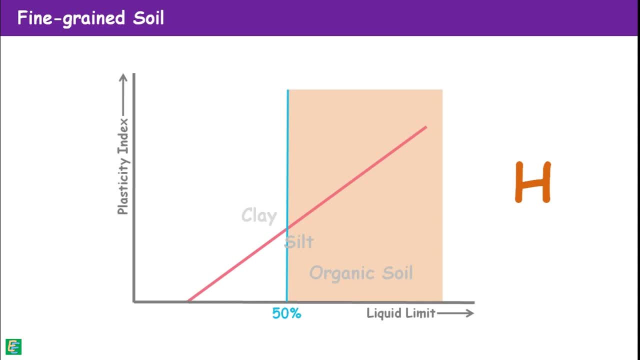 liquid limit and are represented by symbol H. If the soil in this part is clay, then symbol used will be CH, If it is silt, then MH and for organic soil it is OH. Soils lying to the left of this 50% line have low value of liquid limit. 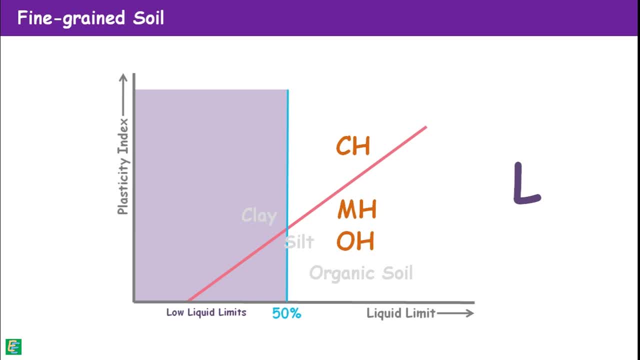 So they are represented by symbol L. Soils in this part are described similarly: CL, ML and OL. This line already separates clays from soil, From silt and organic soil. Now, to distinguish between the silt, which is inorganic soil, and organic soils we use. 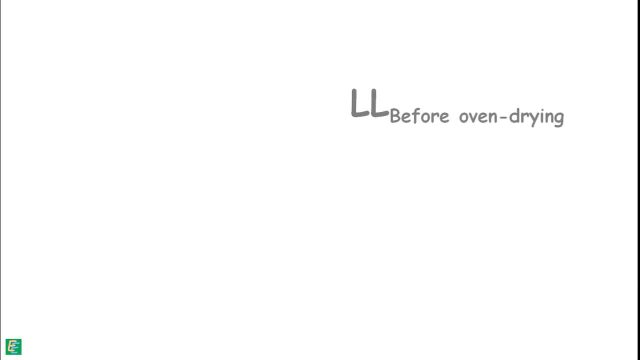 oven drying. We note down the soil's liquid limit before and after oven drying. If oven drying decreases the liquid limit of soil by 30% or more, the soil is organic And it will have symbols OL or OH, And if the decrease in the liquid limit is less than 30%. 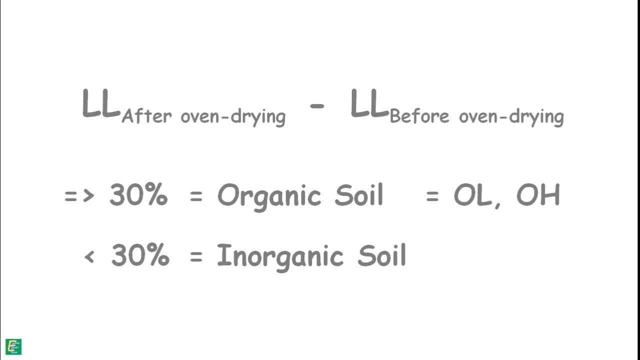 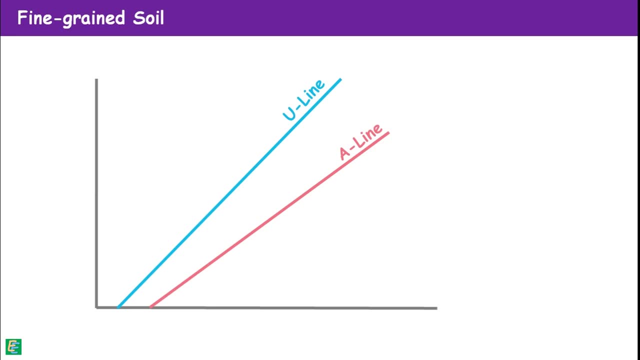 Then it is OH. Soil is inorganic and the symbols will be ML or MH. A U line is also defined as the upper limit of the correlation between the plasticity index and liquid limit of soil. If the test results of the soil fall above U line, then results are considered faulty. 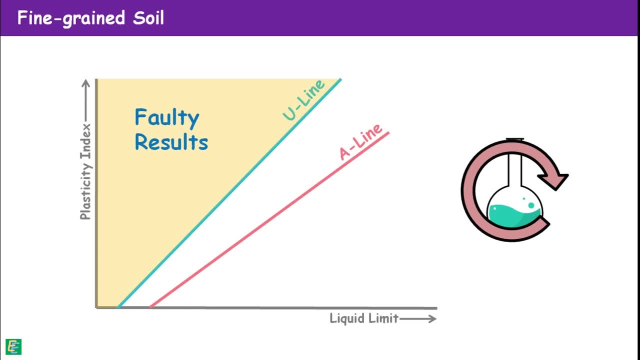 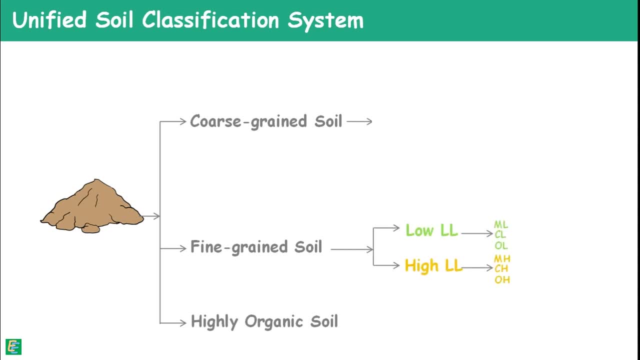 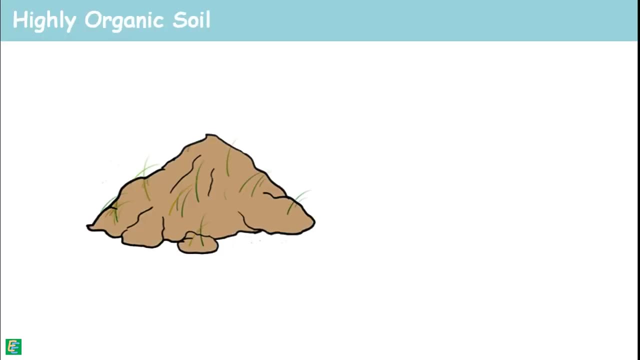 and experiment should be repeated. Equation of the U line is given as this: It was the classification of fine-grain soils. Lastly, the third category unified system defines is highly organic soils. We can identify them by simply looking at them. These soils are termed as peaked and are designated by the symbol pt. 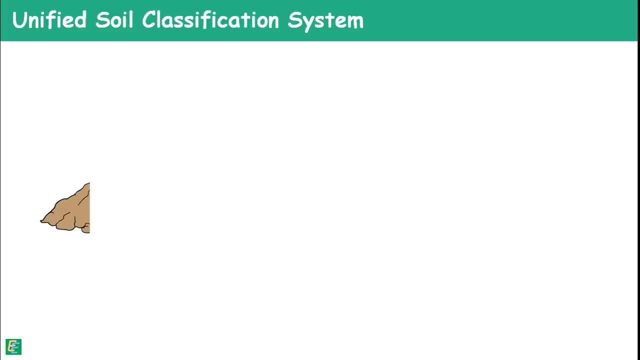 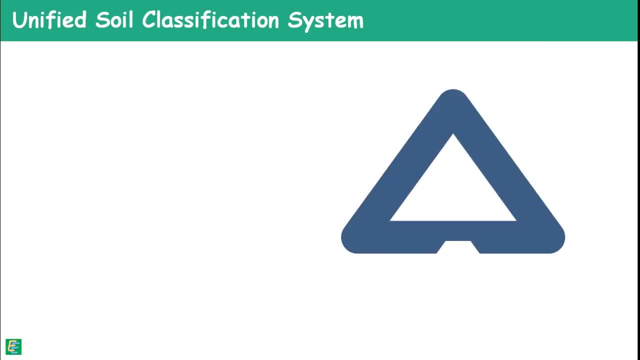 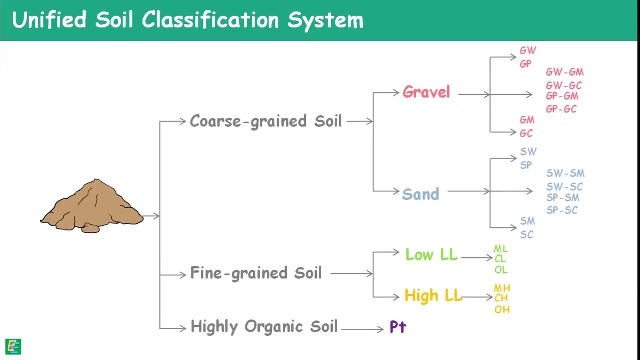 And are more easily defined. This classification system has also been adopted by the bureau of Indian standards, making the Indian standard soil classification system. Indian classification system is in many respects similar to the unified classification system. There is one basic modification, which is in the classification of fine-grain soils. 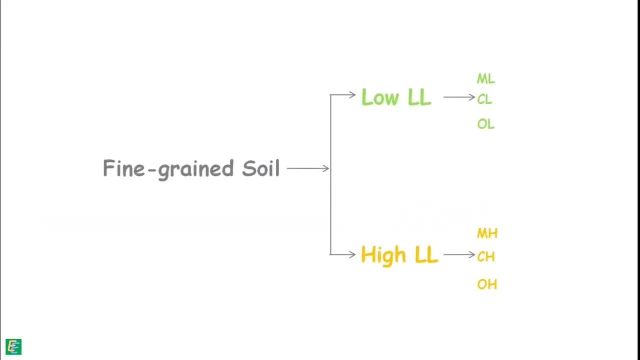 In Indian classification system, fine grain soils are divided into three categories of low, medium and high liquid limit, instead of only two categories of low and high liquid limit in the unified system. Medium category is defined between the liquid limit 35% to 50%. 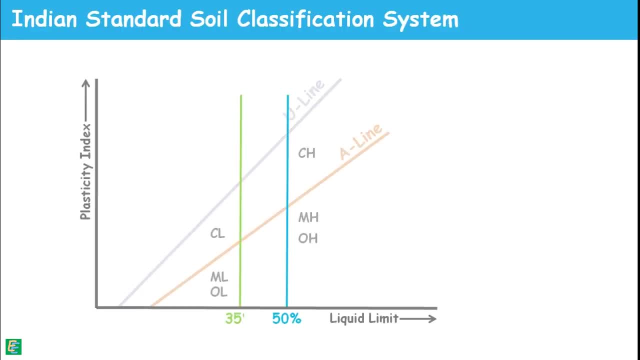 So in the graph another vertical line can be drawn at liquid limit: 35%, and soils falling in this region are denoted by symbol I I. for intermediate such as Ci, Mi and OI, The classification criterion for the coarse-grained soils is the same as the unified system. 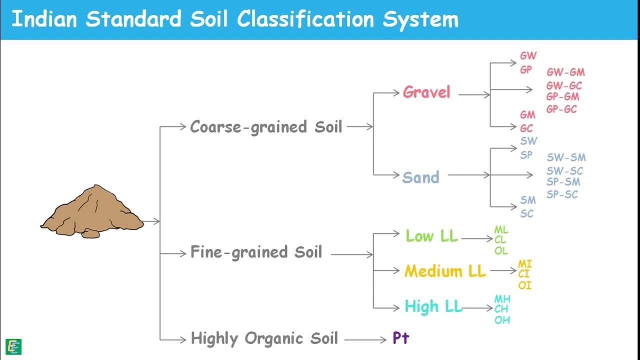 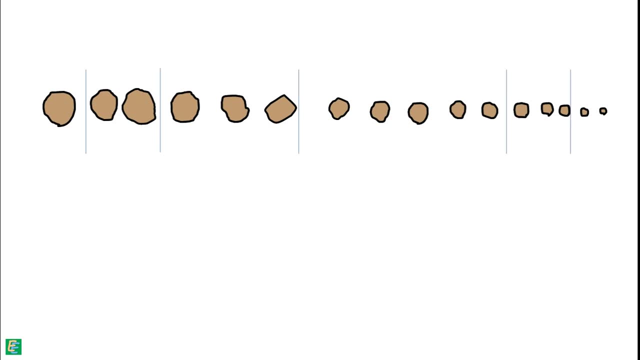 It has similar naming processes. The division of soil fractions purely on the basis of grain size can be shown as this: Soil particles of size greater than 300 mm are based on grain size. These are called boulders. Particles between 80 to 300 mm are called cobbles. 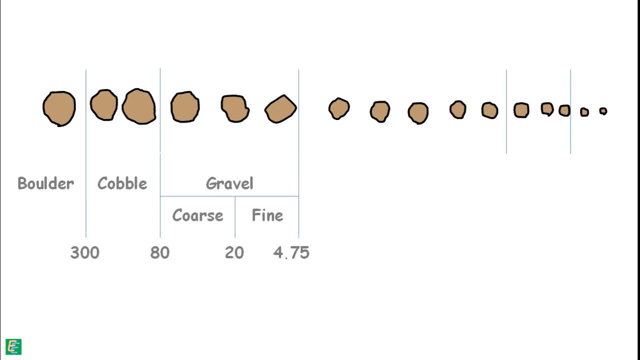 Gravel is defined between 80 mm to 4.75 mm. Sand ranges from 0.075 mm to 4.75 mm. Silp particles have size between 0.075 mm to 0.002 mm, And clay particles are of size below 0.002 mm or 2 micron.